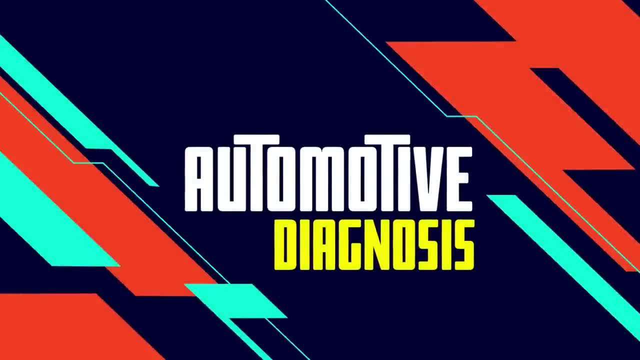 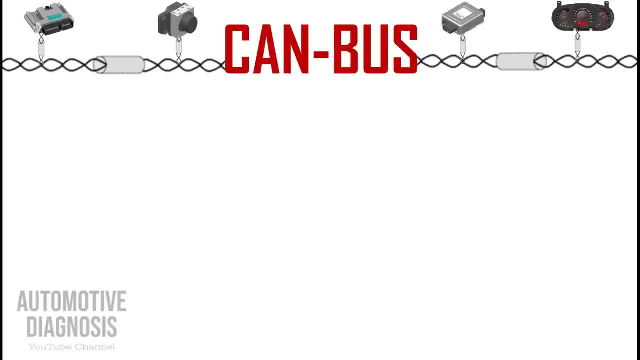 Hi everyone, welcome to Automotive Diagnosis YouTube channel. Today I'm making this video to explain everything needed to understand and to inspect and repair the CAN bus in the cars, Because I've seen many questions about the CAN bus. First of all, for understanding the CAN bus basic itself and how to inspect the CAN bus. So in this, 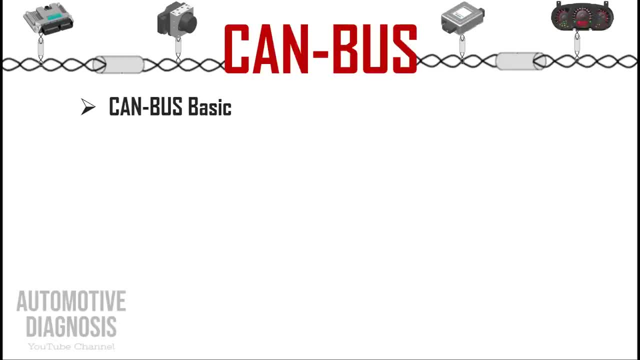 video. I'm going to start from the CAN bus basic, So I will explain how many types of CAN bus we may have in the cars and how these CAN bus are connected to the control units or to each other, and how you can find it in the car as well. 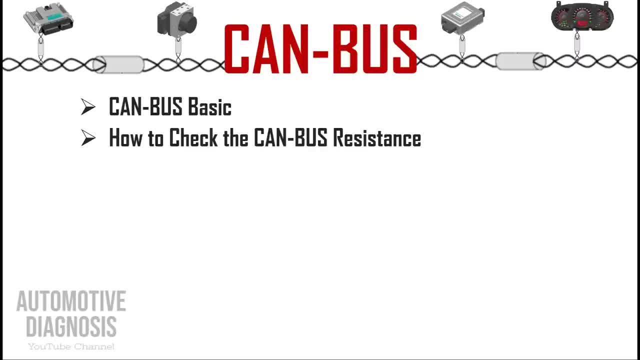 After understanding the CAN bus itself and the structure of the CAN bus, we will see how we can check the CAN bus resistance. Then we inspect the CAN bus voltage and we're going to do this to only with using a multimeter, So it's going to be a quick inspection Then. 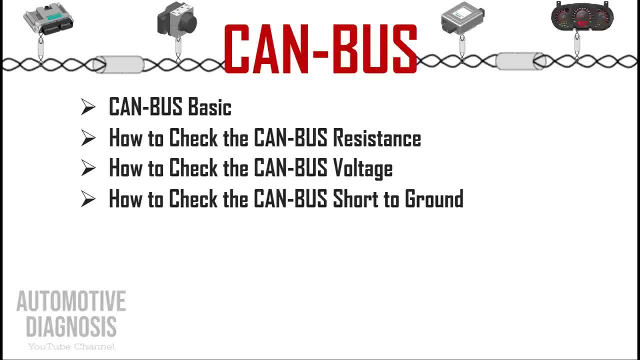 we will see what's going to happen if we have any problem in the CAN bus, like a short to ground, And how we can find it just using a multimeter, How we can find if there is any short to ground in any of the CAN bus. 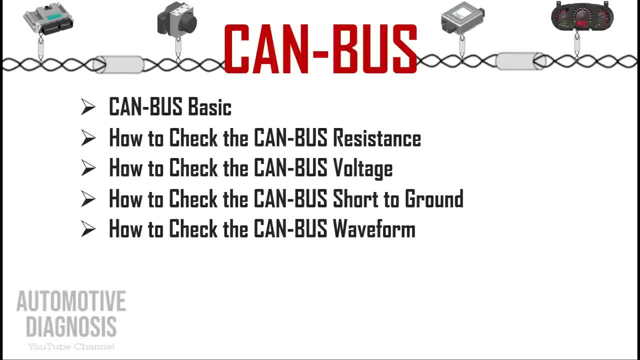 Then we will have a look at the waveform of the CAN bus. We're going to use the picoscope to read the waveform of the CAN bus and we will see if that short to ground happens on the CAN bus. What's going to happen to the waveform when you are reading the waveform. 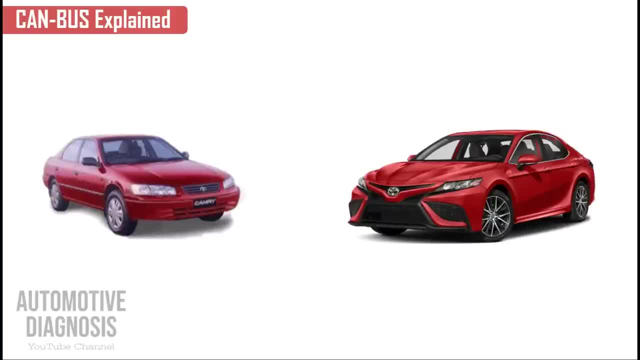 using the picoscope. So first of all, before starting to talk about the basic of the CAN bus, it's really important to know why do we need to have a CAN bus? First of all, if you compare these two cars, one from 2002 and the other one on the right is 2023.. They are both same cars. 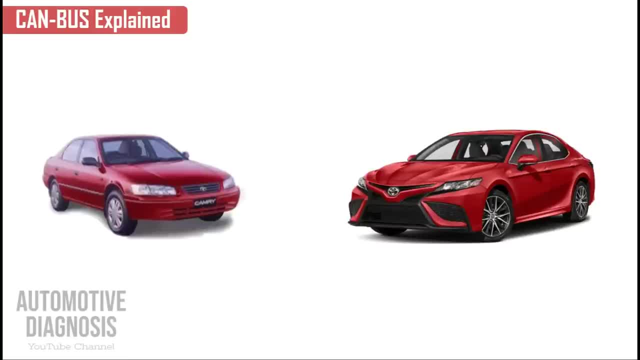 They are Toyota Camry. But comparing these two, what's going to tell you? Obviously, comparing these two cars is not going to be a big deal, But if you compare them, you will see that they are both same. So how many new technologies do you need to use? 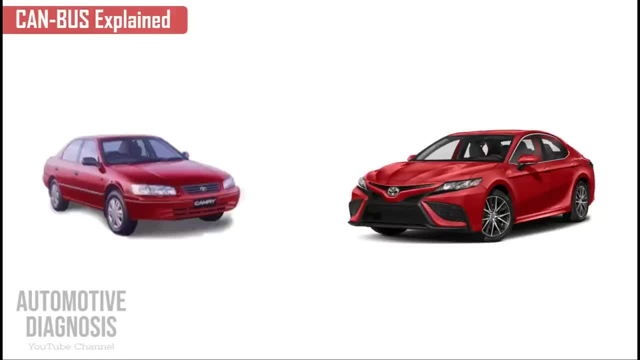 The first thing which is going to come to our mind is how many new technologies we are using right now on the new model. So obviously the new model doesn't have only the external features. It's going to have so many electronic control units, so many new systems and new. 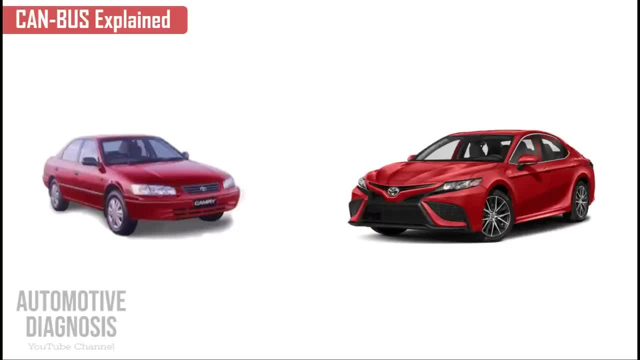 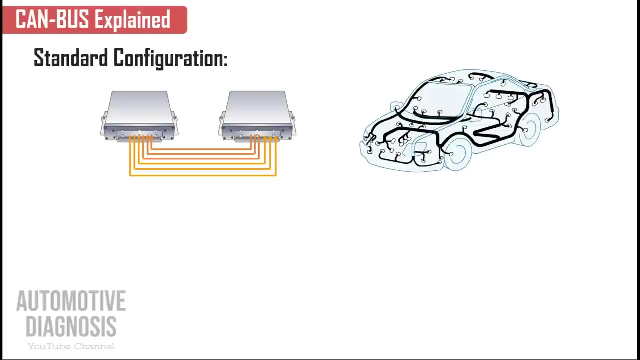 technologies and obviously so many wiring and so many connectors. If we just use the conventional way To connect all these control units together, what's going to happen to all those wirings? This is the standard configuration if we just use the normal hard wire for sending any signals. 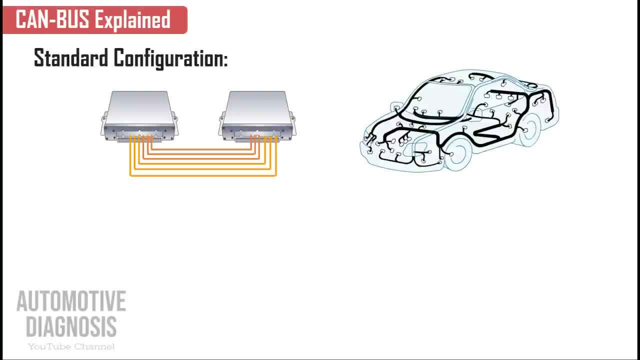 between the units. All right, so what's going to happen? We will have too much wiring, We will have so many connectors and, believe it or not, many problems on the electronic systems And when it comes to repair any electronic system, having so many wiring and so many. 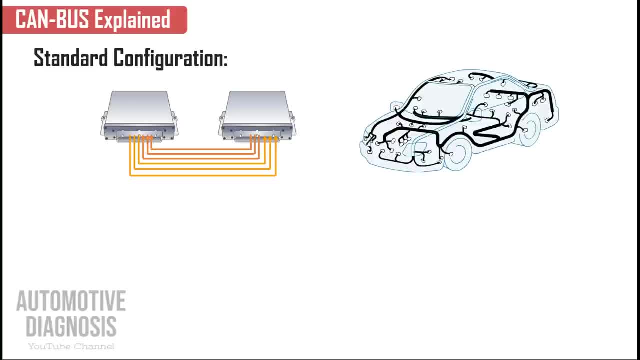 connectors is going to make our life so much harder. So instead of using a standard configuration, we need to find another way to minimize this wiring as much as we can. So the best solution was using a CAN bus, which is a network to minimize the wiring as much as we can. 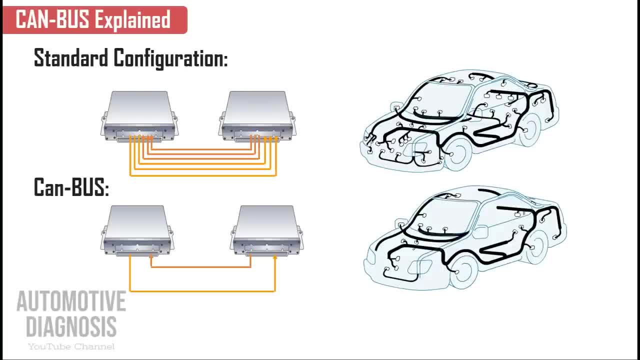 As you see, in the CAN bus configuration we have way less connectors when we compare it to the standard configuration. When I compare these two, I'm not trying to say that we don't have any hardware connection anymore, We just have the CAN bus. No, of course not. But CAN bus is there to minimize. 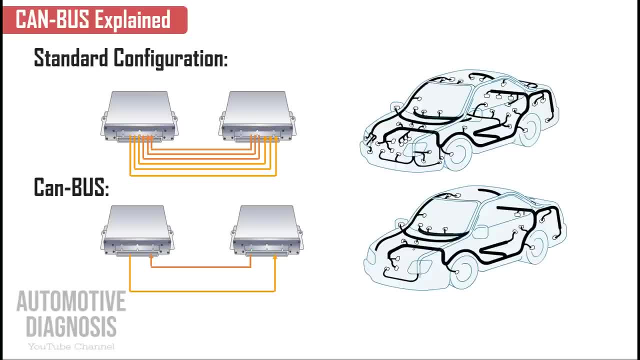 the need for having all these wiring. So it means If if we need to send one signal to multiple units, we don't need to use many hard wires to send this signal individually to any control unit. we can just use the network to share it with other control units. 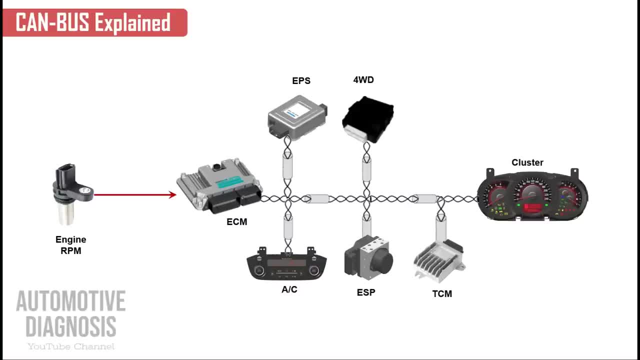 for example here. so if you look at this configuration, you will understand what i'm trying to say. so what you see on the left, right here, this is the crankshaft position sensor which is going to send the engine rpm signal to engine control module. so obviously we have 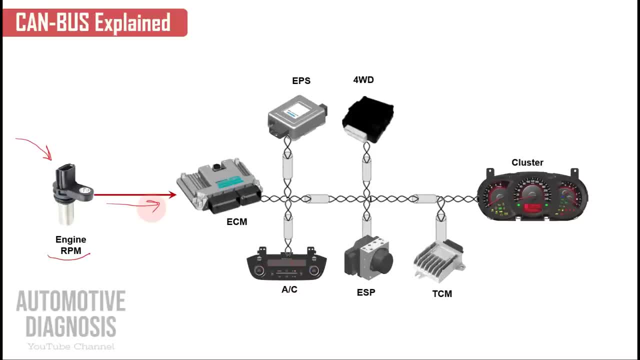 some other control units which need the engine rpm signal. but do we have multiple crankshaft position sensors? no, we don't. we only have one. so it means we only have one crankshaft position sensor to read the engine rpm and send the signal to engine control module, which we call it. 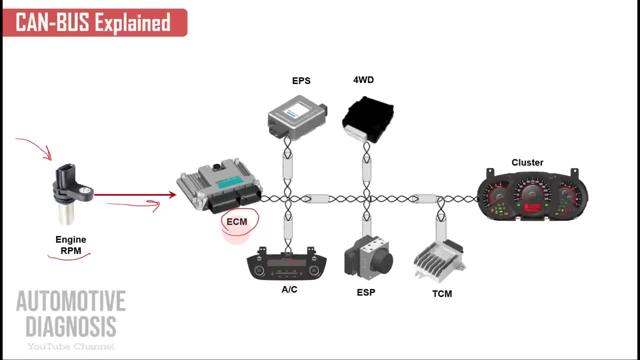 ECM here. so what's gonna happen for other control units that need the engine rpm signal? I'm gonna just mention some of them, because there are so many units, so many control units that need the engine rpm. for example, right here we have EPS, electronic power steering, which needs the engine rpm signal to to know. 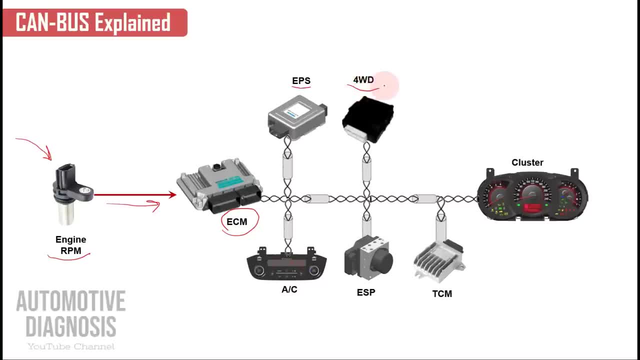 when engine is started. we know the four-wheel drive system. we have the air con. air conditioning also need to receive the engine rpm signal. we have ABS or ESP and we have transmission control module as well, and what we have on the right is the instrument cluster. obviously, this unit needs the engine rpm. 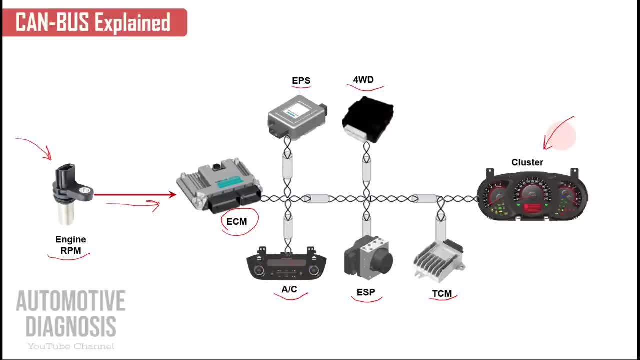 as well to to show the engine rpm to the customer. so in this case, instead of sending the signal individually to all control units, what's gonna happen? ECM is gonna share the information using the network. so what you see right here, this is actually representing the network and ECM is gonna send the engine rpm using this. 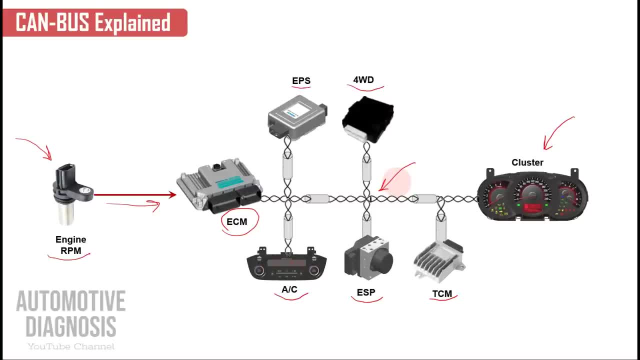 network to all these control units so we don't have individual wires for each single signal. and this is only one example, because there are many signals that you seem needs to share with other control units and obviously other control units need to share some information with with some. 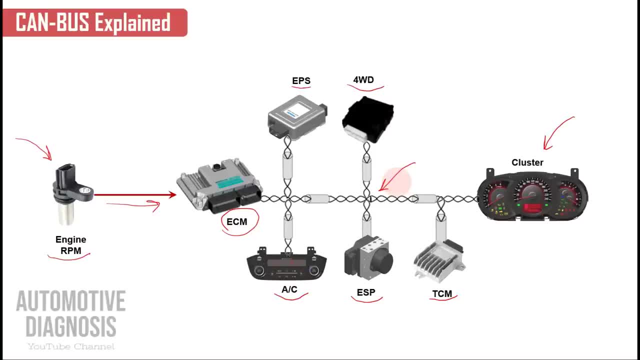 other units as well. so what's going to happen? instead of having so many hard dem pour de la direction ang ON, roud, roud onward. these control units like uh electronic power string. this one can send the information uh through the canvas. it can share the information through the canvas for all other control units. 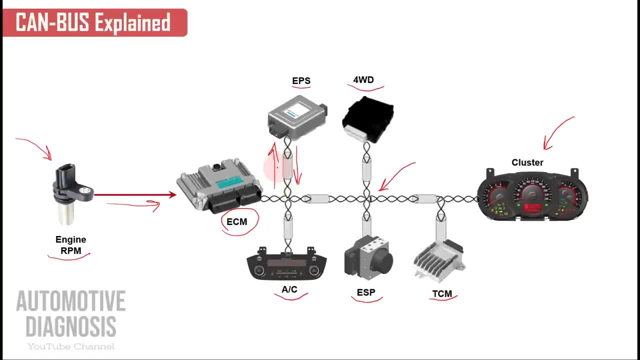 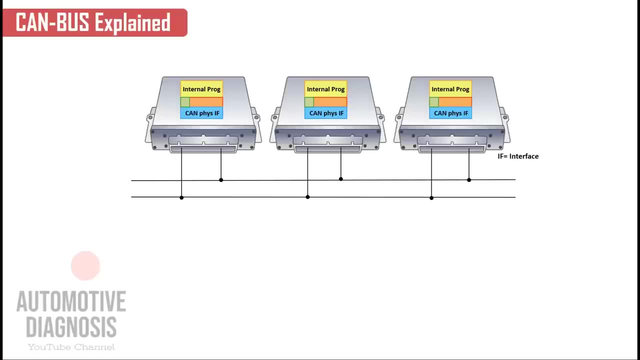 or it can receive the information from the canvas. so you see how how much this configuration is going to minimize the need for wiring and for connectors. uh, so let's talk more about the canvas itself. let's see how these control units are connected to the canvas. so generally, as you see here, all the control units are connected in parallel. 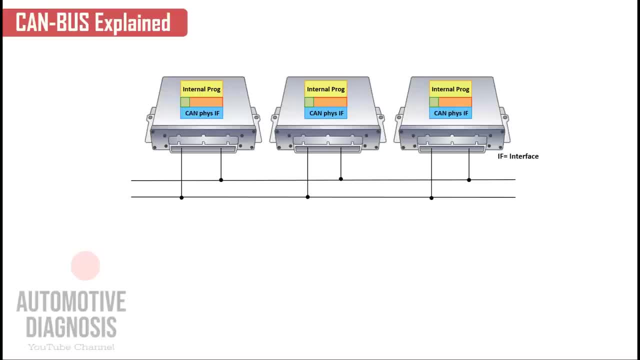 to the canvas. so it means canvas is a multi-master network. it means if something happens for one of these control units, canvas still is going to work. so we can say canvos is a multi-master network. it means every control unit in a canvas can send and receive information individually. 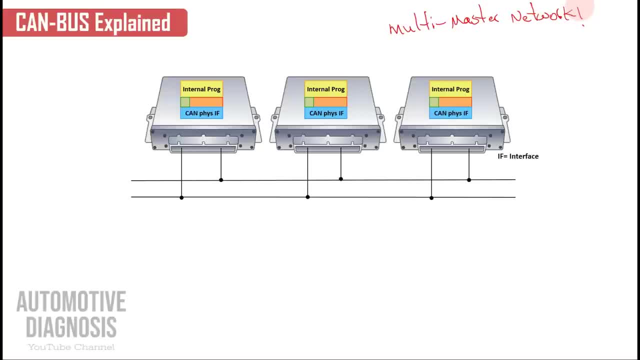 so do we have any other physical control unit externally that we can find and we can see and we can say this is actually the CAN controller? No, because the CAN controller is built inside any control unit which is connected to the CAN bus. So what we see here, CAN physical interface. 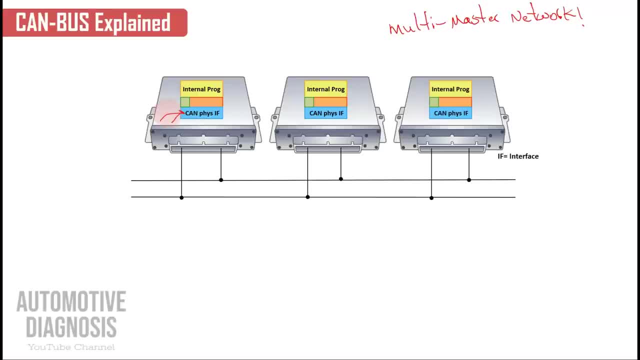 So this is the CAN physical interface. So it means the CAN IC is actually installed inside any of these control units. So it means if this control unit receives any signal from the CAN, this CAN physical interface is going to receive the information, is going to convert it to. 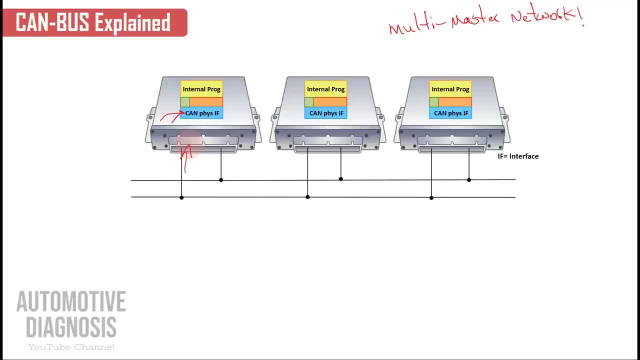 a message that internal program of this ECM can read, and then it's going to send it to the internal program. Okay, so all control units are like this one, So you don't see any physical control unit that you can point at and you say: this is the. 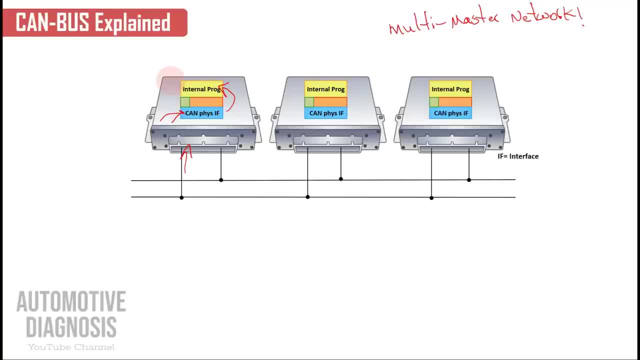 control unit. So you don't see any physical control unit that you can point at and you say: this is the CAN controller. No, the only thing you see is just a normal control unit inside the car and these twisted wires, a pair of twisted wires, which actually represent the CAN. 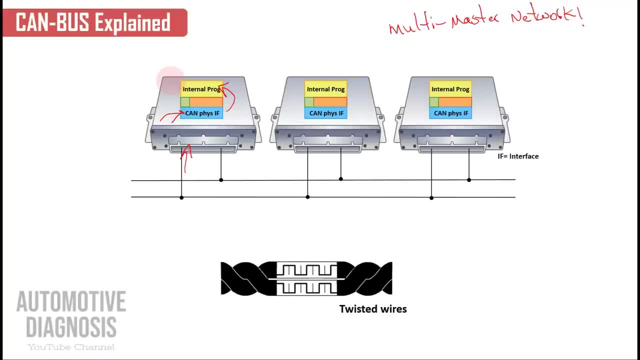 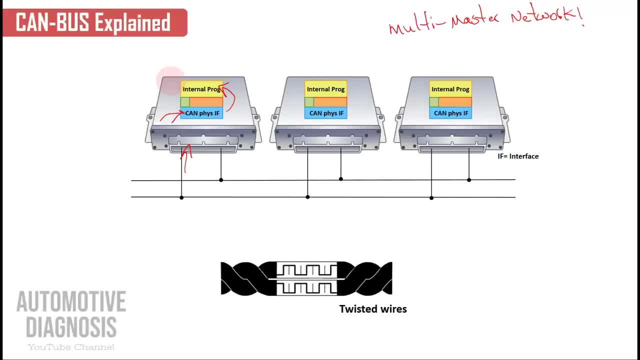 called CAN high, the other one is called CAN low. So between these two I can say: this one is CAN high and the other one here is CAN low. So what do I mean by saying CAN high and CAN low? Am I referring to high speed and low speed? No, 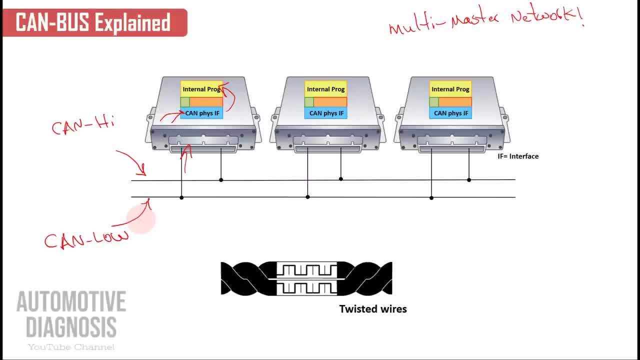 not at all. Yes, obviously we have high speed CAN, we have low speed CAN, we have different classes of the CAN that each one of those classes is going to give you different speed. But here, when I say CAN high and CAN low, 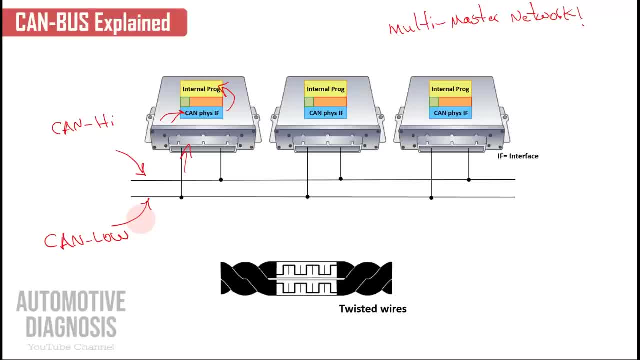 I'm not referring to the high speed or low speed, But between these two twisted wires. they have different voltages. So when I say CAN high and CAN low, I'm actually representing to each of these two wires, because one of them is going to give you higher voltage, the other one is going to give you 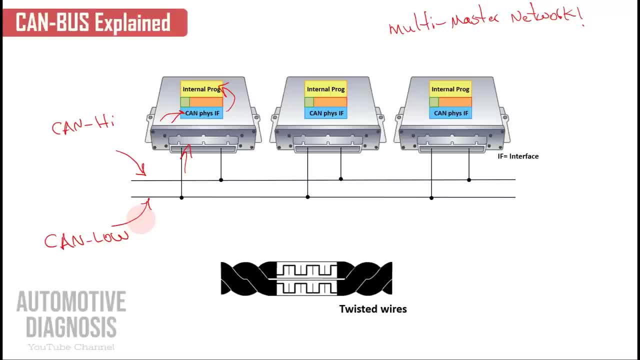 lower voltage. So when CANboss is functioning, the voltage on CAN high is going to change from 2.5 volt to 3.5 volt. So this is the voltage on CAN high. But what about on the CAN low? On the CAN low. 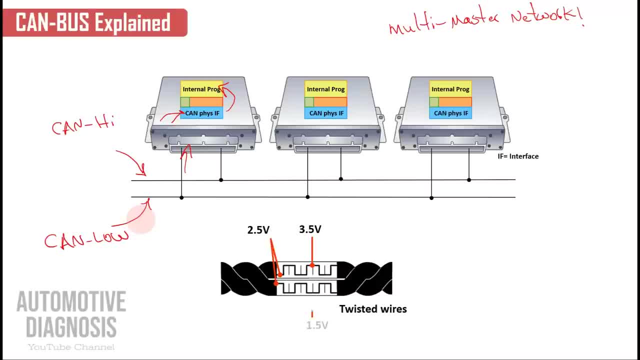 voltage is going to drop from 2.5 to 1.5.. So this is actually the amount of voltage that we can receive and we can measure on the CANboss. We will see how we can measure on the CAN low. We can inspect and how we can measure the voltage using a multimeter and using a picoscope. 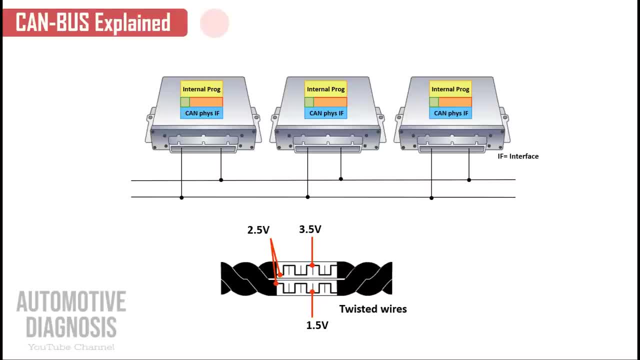 So it's really important to know that what we are talking right now about the CANboss, it's actually the high speed CAN which is normally sometimes is called C-CAN. Okay, so this high speed CAN has all these features because this voltage that I told you. 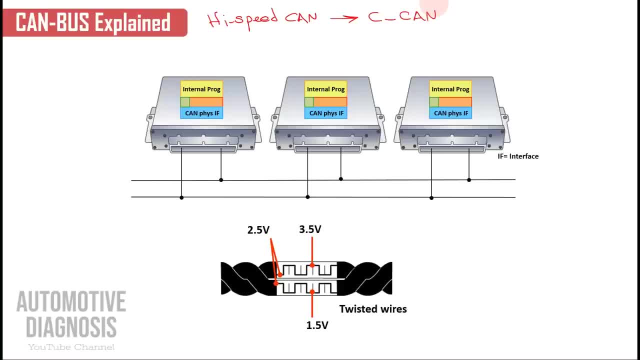 it's only for the C-CAN. When we are talking about the different type of CAN, like body CAN, this voltage is going to be different. So this voltage, it's only for C-CAN. Okay, so what is the speed? It's only for C-CAN. 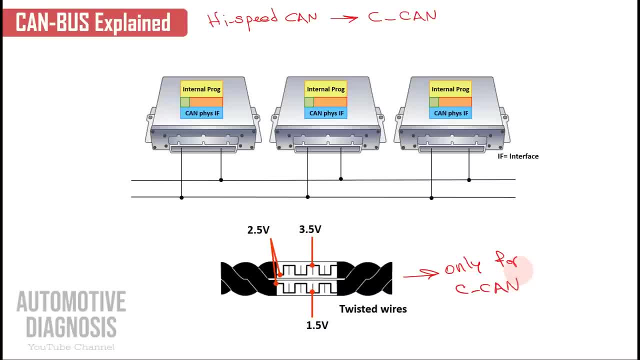 Okay, so what is the speed? It's only for C-CAN. Okay, so what is the speed? It's only for C-CAN. The thing specific about this C-CAN is actually the speed. So normally this class of the CAN. 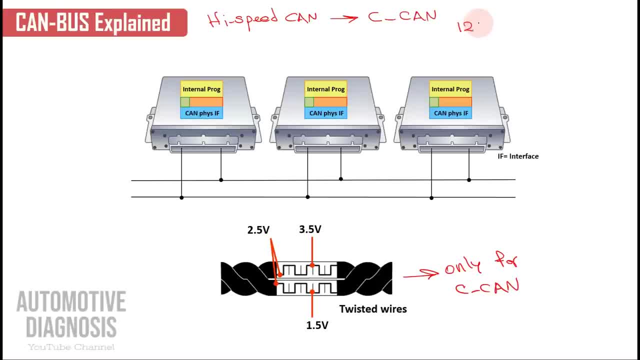 is going to give you this speed between 125 kilobit per second to 1 megabit per second. This is actually the other advantage when we are using the network, Not only we are using less wiring, less connectors and troubleshooting procedure is going to be much easier, but also. 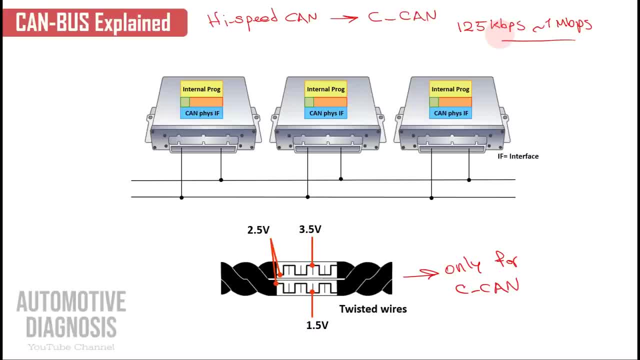 we are transferring the information much, much faster, which is gonna make all these systems more reliable. all right, we already know that we are talking about the ccan and, as you see, all the control units in the ccan are connected to can high and can low in parallel. but we need to. we 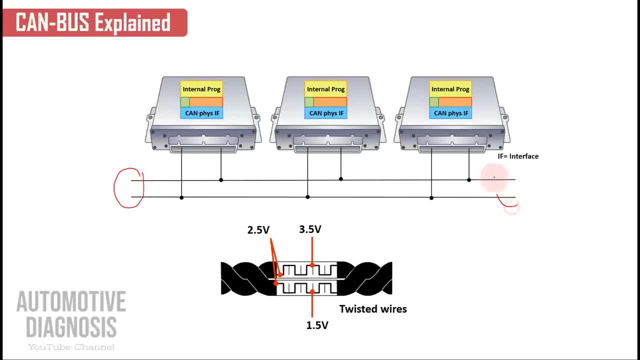 need to think about these two point of the circuit as well. obviously we cannot connect these two circuits together to make a full parallel circuit, because these two wires, each one of them has different voltage, because one of them is the can high, the other one is a candle. 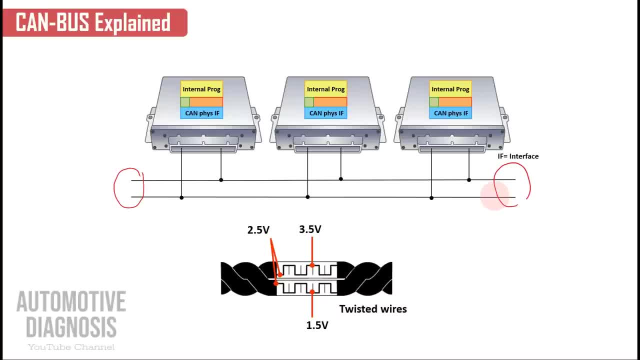 and, on the other hand, if we don't connect these two together, what's gonna happen? we won't have a parallel, we won't have a full parallel circuit. we need a parallel circuit to stabilize the voltage, otherwise a serious problem is gonna happen to our issues. so what's? 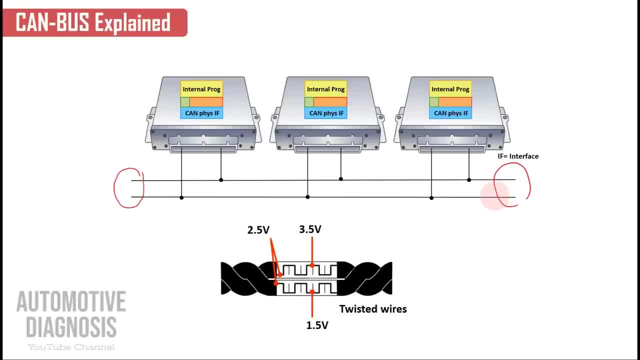 gonna happen? how can we connect these two lines together without having any problem? so what we have here? we have terminating resistor one to any, all on each end. so what's gonna happen? by having these ones, we won't have any other problem for connecting these two lines together. it's really. 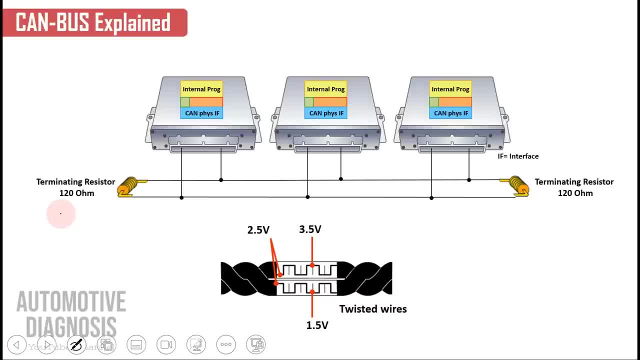 important to remember that these two terminating resistors only used on ccan. so if you're troubleshooting the body, can, you won't have the terminating resistor anymore. so where are the locations of these terminating resistors? normally most of the time? uh, this one, most of the time is. 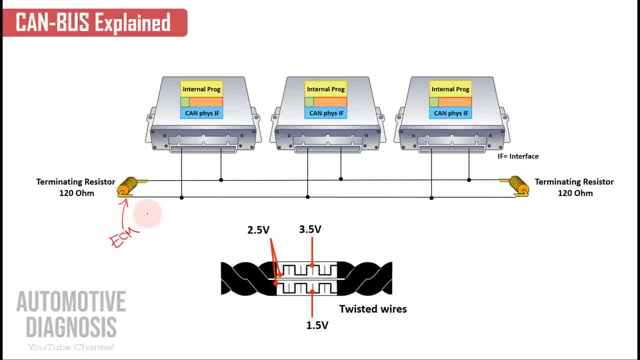 inside the ECM. so I haven't seen anything different on most of the cars I've seen of one terminator 1953, a store is installed inside the ECM and i have current tickets and the other one is currently ecm. but what about the other one? the other one can be different. i've seen many different cases. 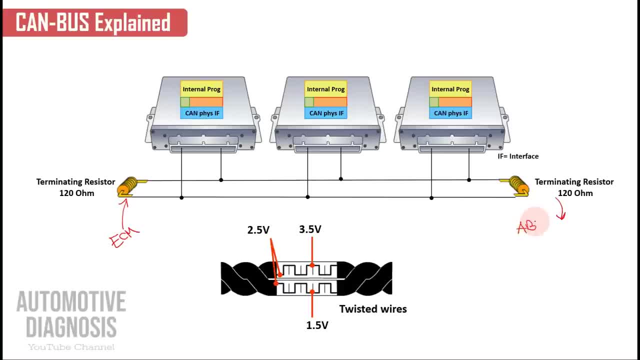 for the other one, sometimes it's uh inside the abs or uh esb module. sometimes it's inside the instrument cluster. i've seen i've seen that sometimes inside the interior fuse box, ip junction box, uh, and sometimes it's an external uh resistor. so for for for finding this one, you 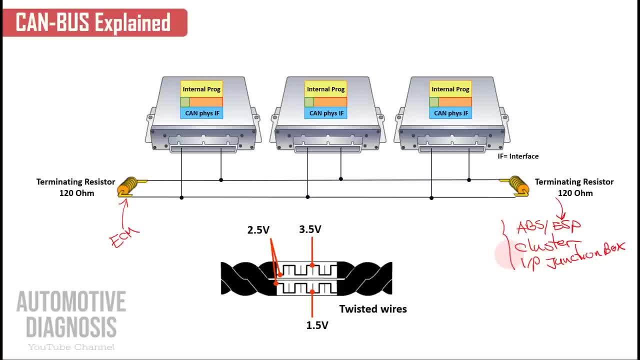 need to have a look at the wind diagram to see, uh, where's the location of the terminating resistor. but i'm gonna uh explain how uh you can measure the total resistance for uh for the canvas. so, as far as we know, we have two uh terminating resistors, each one 120 ohm, and we know that. 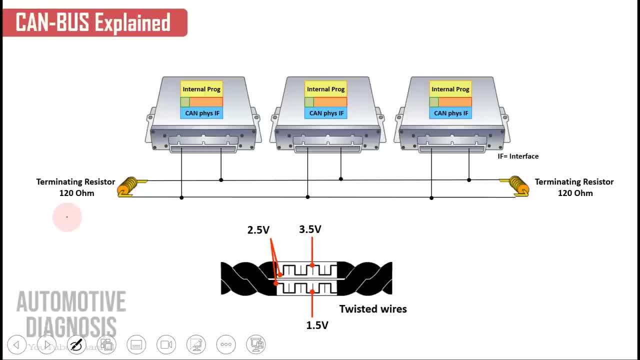 this circuit is full parallel circuit. so later on i'm going to explain how to inspect and how to measure the canvas resistance. but it's really important to know what's going to be the total resistance when you are measuring. so this one is actually a parallel circuit, so for checking the total resistance in a parallel 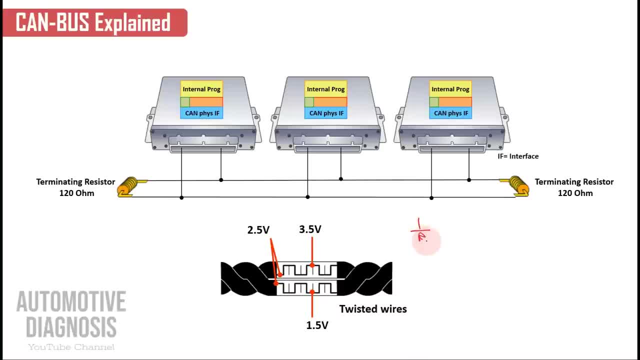 circuit. we need to just use this formula: one by our total is going to be equal to one by r1. one bond, one by r2. okay, so here we have r1 and r2. these two are referring to the terminating resistor, so we can say 1 by 1. 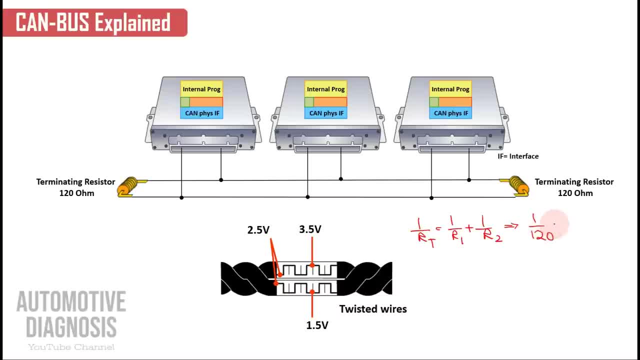 2 bande register by 120 plus one by 120, right? so it's going to be like this: one by our total is going to be 2 by 120, which is going to be 1 by 60.. okay, so the total calculation is going to be. 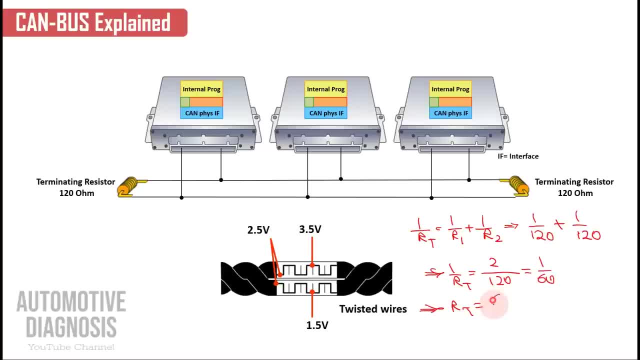 our total is going to be something close to 60.. so this is what we are after. okay, so when we are checking the canvas resistance, we are actually going to measure something close to 60 ohms, and i'm gonna show you guys how to find the inspection point and how to measure the. 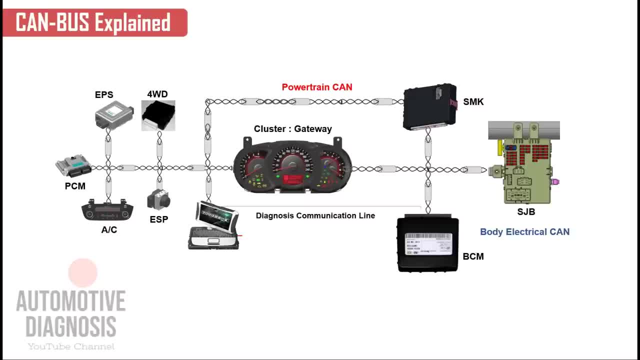 measure. so i already told you that we have the C-CAN or powertrain CAN. so some control units like the engine control module, transmission control module, four-wheel drive, electronic power string, aircon, abs, esp and instrument clusters, all these units are connected to the c can. we may have some other. 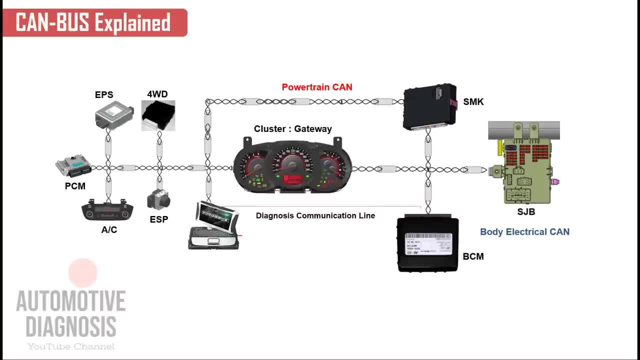 control units as well, because right here I'm not referring to all the control units, because each different car may have more or less control units, but on the other hand we have some other, some other classes of the can as well. like the body can, so body can normally is used for communication between some control units. 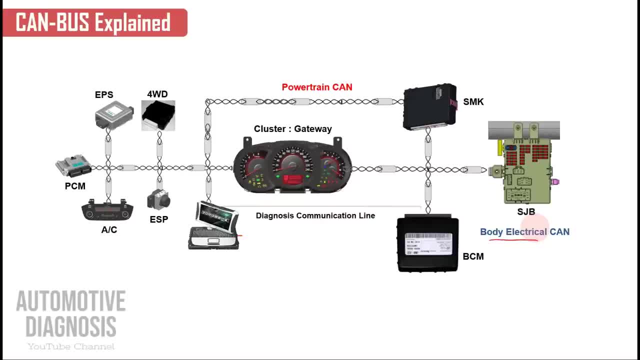 inside the car and and normally is going to give you less speed. between these control units, you may see some of them which are connected to two different type of cans, for example, instrument cluster, so this cluster is connected to C can and body can at the same time. or this one smart key control module in 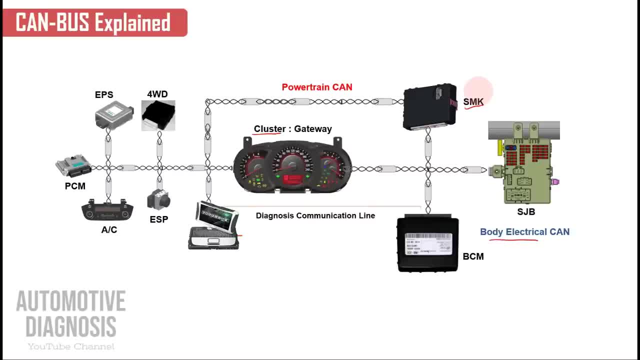 this case is connected to a power train can and body can, but between these ones sometimes we have some control units that are connected to the instrument cluster. so we have some information that must be sent from one unit in that C can to another unit in the body can, for example the reference for vehicle SP. 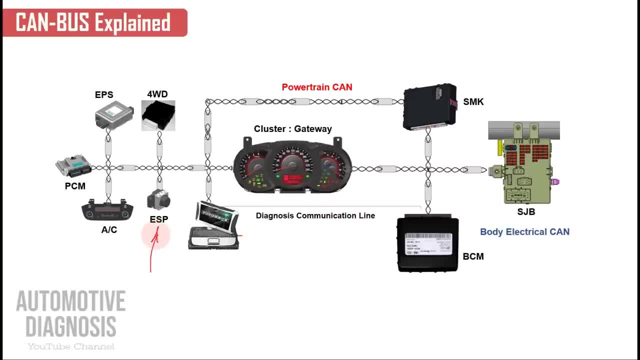 signal is ABS and ESP control unit, but some other control unit, like the BCM body control module, might need this information as well, for example to lock or unlock the doors automatically. so what's gonna happen? BCM is connected to the body can, but ESP is actually on the C can, so these two don't 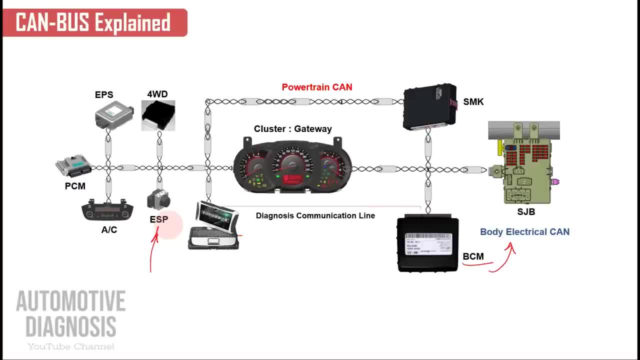 have any direct connection. so how how can these two control units share the information? that's exactly the time that we have the Gateway. so gateway is actually one control unit which is connected to two different type of can to share the information between them. so it means When vehicle speed signal is needed on BCM, ESP is going to send the information of the vehicle speed through the CCAN to instrument cluster. 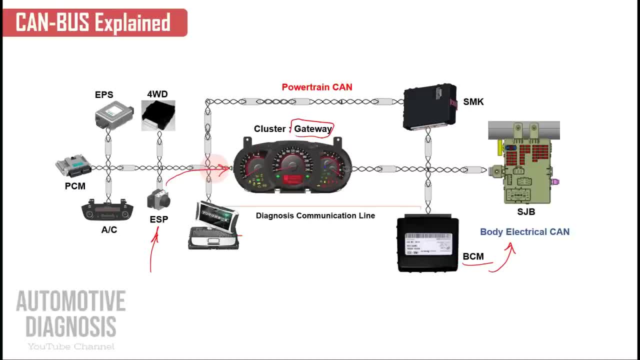 So cluster is going to receive the information in a CCAN, then it's going to confirm it to another format for BCAN and it's going to send it in the BCAN. So cluster is going to work as a gateway to receive the information from one unit in a CCAN and convert the signal to a BCAN to send the information to that control unit. 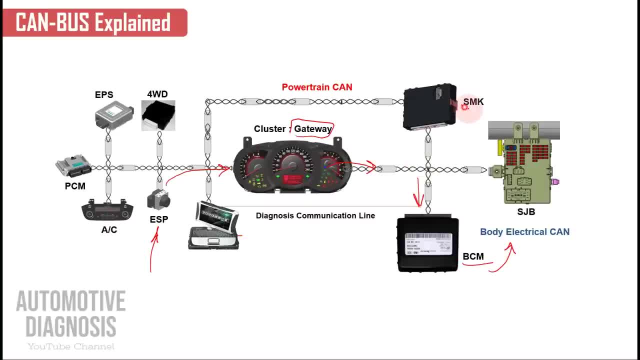 So, as you see, as I said earlier, smart key control module is connected to CCAN and BCAN as well at the same time, But this one is not. this control unit is not playing a gateway role. Gateway in this case is on the instrument cluster. 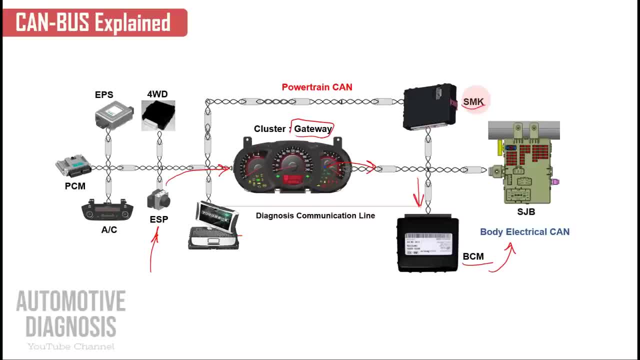 Even if a smart key control module is connected to CCAN at the same time, that one is not going to play a gateway role. The other important item is actually this one, which is your scan tool. Your scan tool is going to get connected to the CCAN as well from DLC connector. 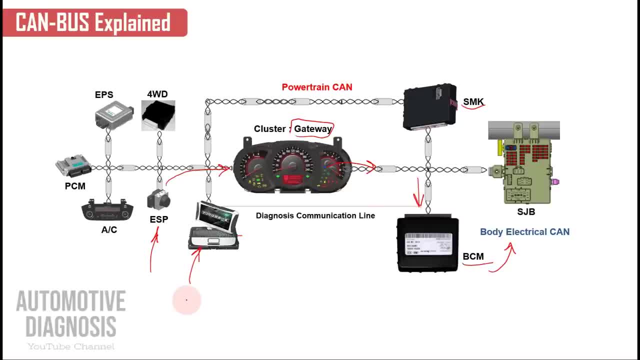 So you have the DLC or OED2 connector which is connected directly to the CCAN to diagnose, To diagnose all the control units connected to the CCAN. So this is really important. but your scan tool to diagnose other control units which are not connected to the CCAN is going to use another diagnosis communication line which is normally sometimes, which is sometimes a K line. 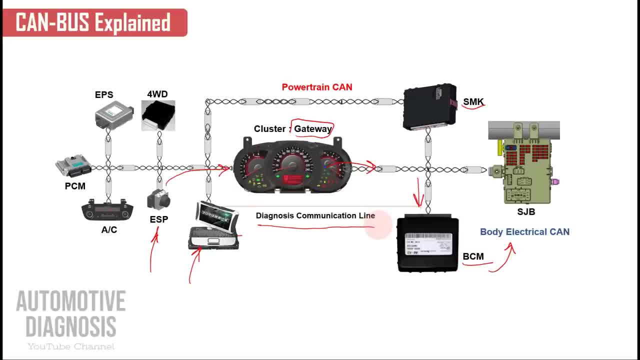 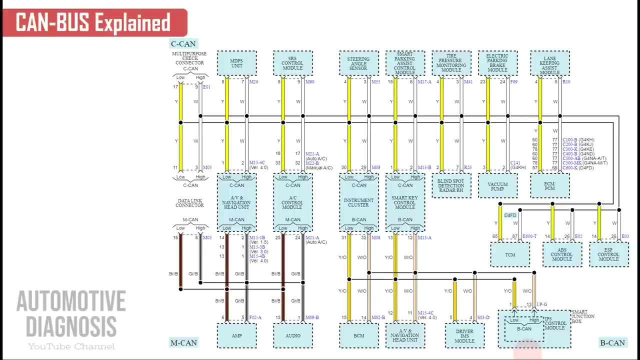 So that's different. For example, in this case, your scan tool is not going to diagnose the BCM using a CCAN. So this, this is really important fact to know. Okay, let's have a look at this one diagram for one card that has three different type of CAN. 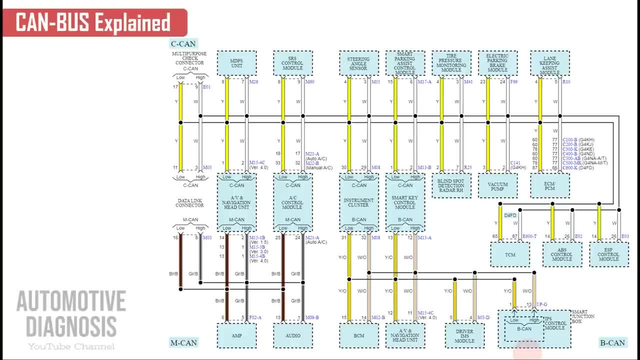 So we will see what control units are connected to each one and we will see the gateway for each one as well. For example, this one is actually CCAN at the top left. So some control units like electronic power steering. We have the SRS or airbag. 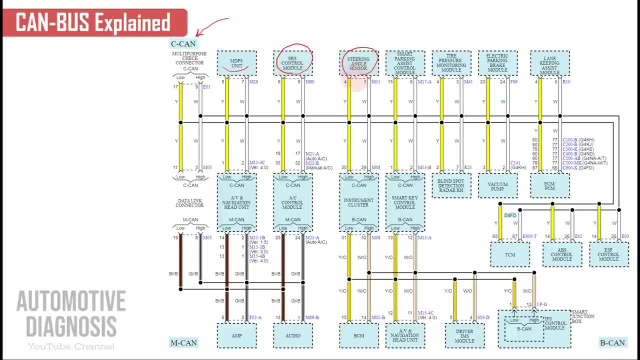 We have the steering angle sensor right here. We have the smart parking assist type version monitoring system- electric parking brake module or EPB lane keeping assist system- right here. We have engine control module right there. In this case, vacuum pump is connected to the CAN bus as well. 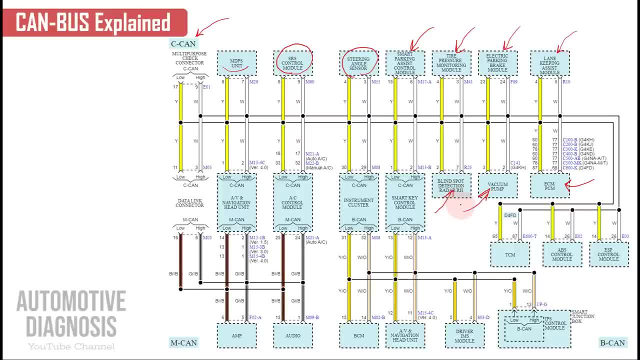 And blind spot detection Detection system as well. So these are the units which are connected only to the CCAN and a couple of other units right down here, like the TCM transmission control module, ABS is right here as well- or ESB- if your car has ESB, obviously ESB is connected to the CCAN. 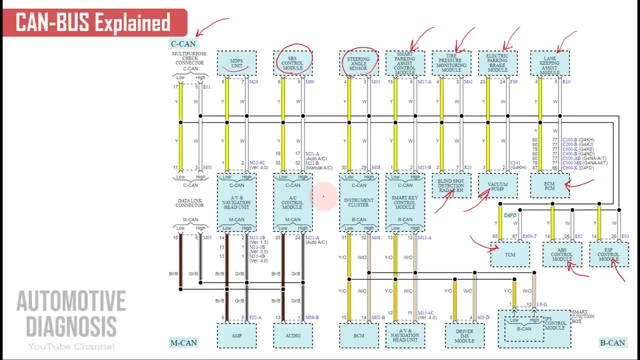 So we have some other control units in between, Like the navigation system, AC panel, instrument cluster and a smart key control module. So these units, all these units, are connected to the CCAN, But between these ones we have we have gateways as well. 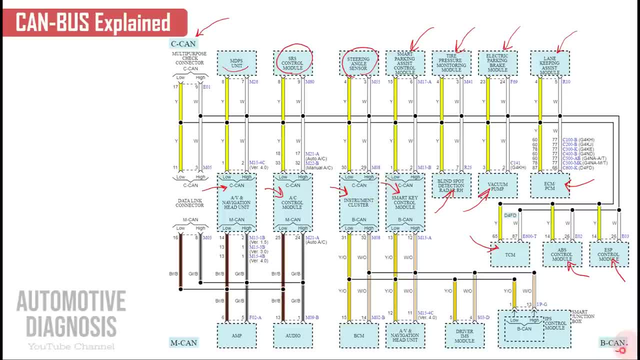 If you look down to the right or to the left, we have V-CAN in here for body CAN and M-CAN right on the left for multimedia CAN. So we have two other CANs here, multimedia CAN and body CAN. 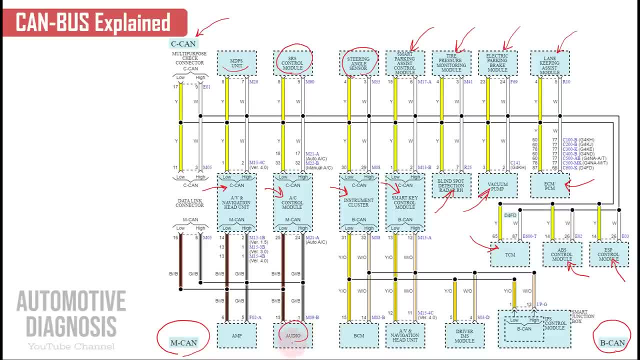 So for multimedia CAN we have the audio system and amplifier. These two are connected to the multimedia CAN And, as you see, we have two other control units, AC control units. So we have two other control units right here and navigation right there as well. 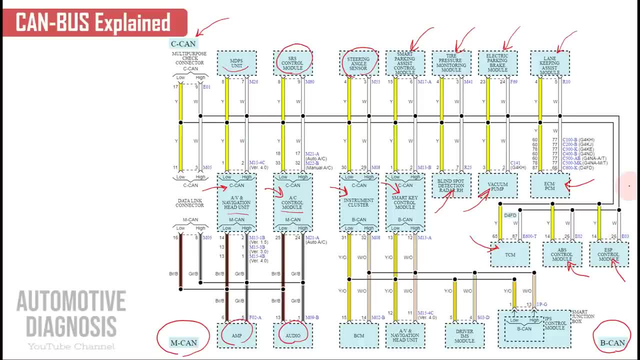 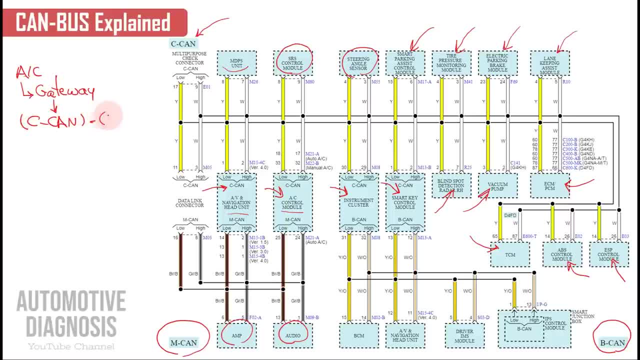 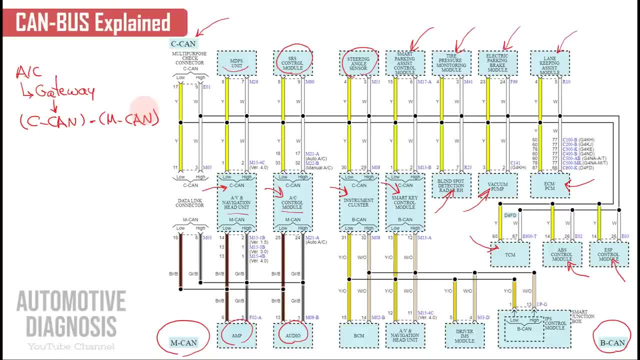 Navigation is not a gateway in this case. But what about for the B-CAN, for the body CAN, For the body CAN? we see the BCM, We see the head unit, We see driver IMS module or integrated memory system. We have the smart junction box as well. 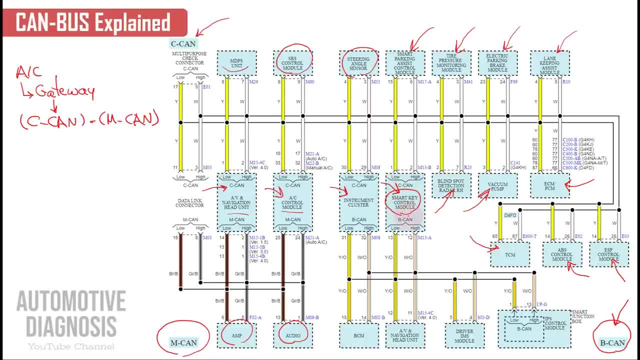 But right here we have a smart key control module- As you remember, we had it in the previous section- And we have the instrument cluster as well, And I explained already that between these two, only instrument cluster is the gateway between C-CAN and body CAN. 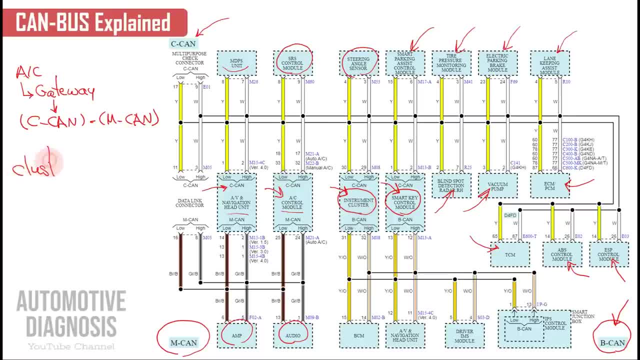 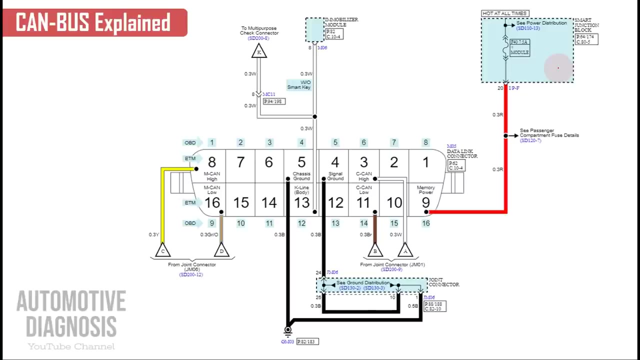 So it's going to be cluster Will be again gateway And And And. Gateway For C-CAN and body CAN And And For C-CAN and body CAN. But how can we reach to the CAN bus? 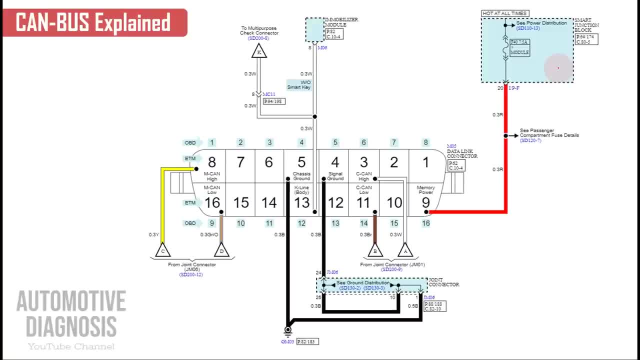 But how can we reach to the CAN bus, the structure to show the gateways? but this one is this. but this video is generally talking about the diagnostic procedure and and the basic of the ccan or high speed. so obviously we need some point to reach to the canvas to measure without having any problem, without actually trying to 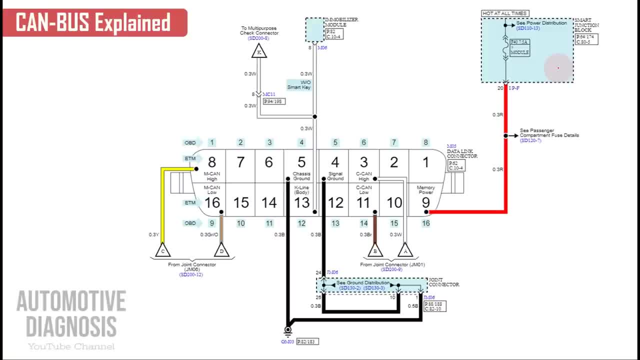 reach to any other section of the wiring when we are trying to do the quick inspection. as i said earlier, your scan tool is going to be one part of the canvas when you try to diagnose the car because when you connect your scan tool to dlc connector. 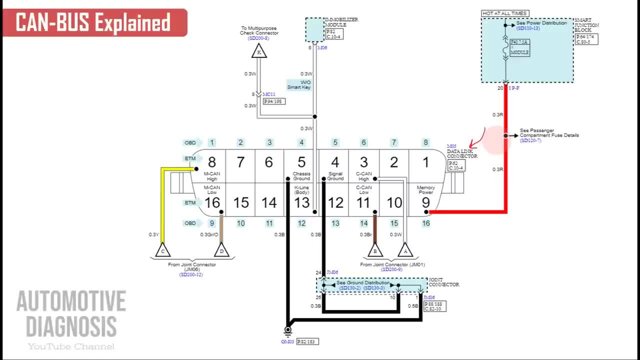 your scan tool is going to be actually one part of the canva, so it's going to send a request for the information and all other contributing needs will be communicating with your scan tool to send the information. so, for finding the ccan high and ccan low, 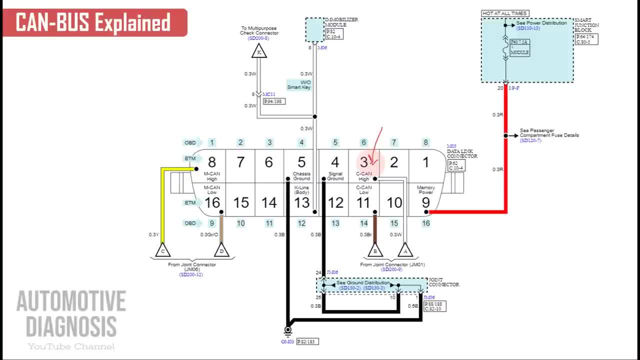 you can just have a look at here: this is the c can high and this one is the ccan low. but, uh, on this car manufacturer, these numbers are just like this: one, two, three, three and 11, four, uh, for the can high and can low. but please, uh, just try to have a look at this one as well, because 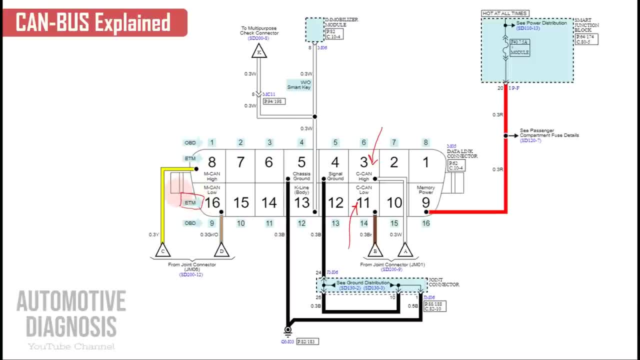 these numbers are only for electronic troubleshooting, manual, whatnot. those numbers that we need are actually the numbers on obd2 itself. okay, so our number is going to be number six for can high, c can high, and number 14 for c candle. so the only thing you need is uh to find the obd2 connector, which is most of the time on the driver. 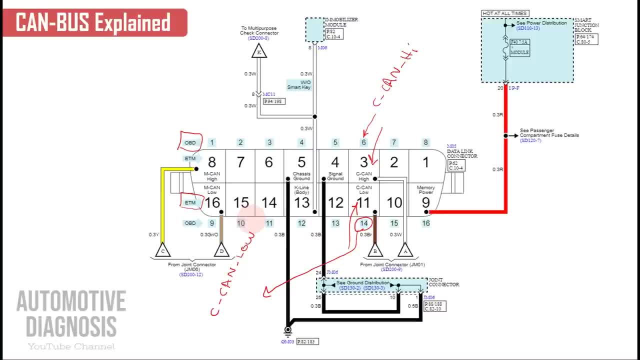 side, find these two pin numbers 6 and 14, and we know that the pin number 6 is going to be for the can and pin number 14 is going to be for the can, low, and the rest is going to be what? uh, i will. 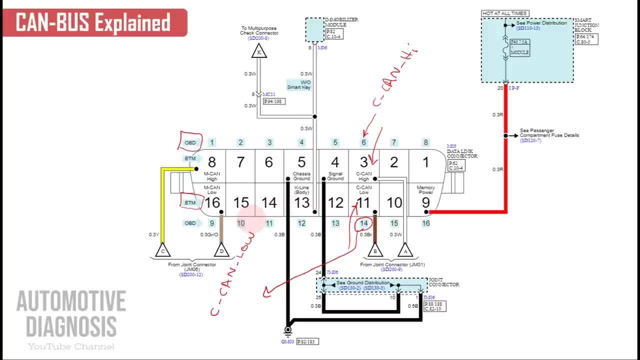 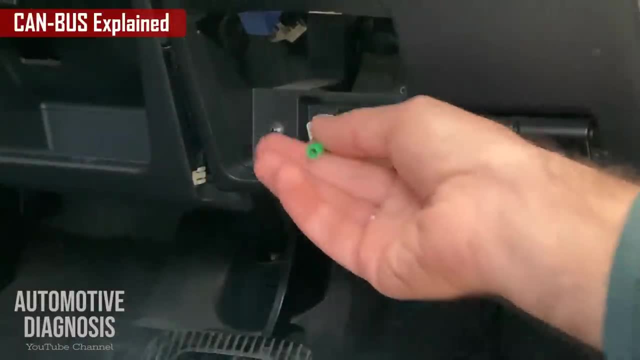 explain to you guys on the car: uh to uh to inspect the canvas release, and the rest is going to be for the can, low resistance, to inspect the canvas voltage and to read the waveform. so the first step for checking the canvas is, uh, to check the total resistance. so, as i said earlier, we can, you can, reach to the. 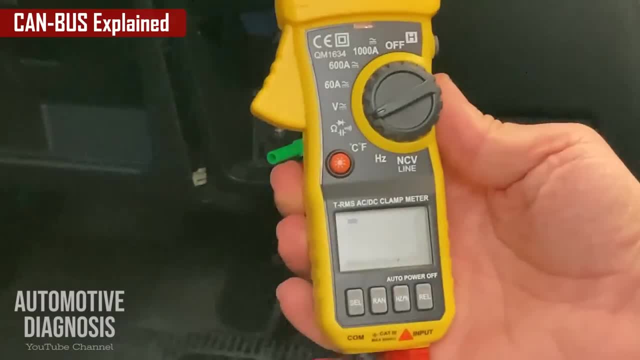 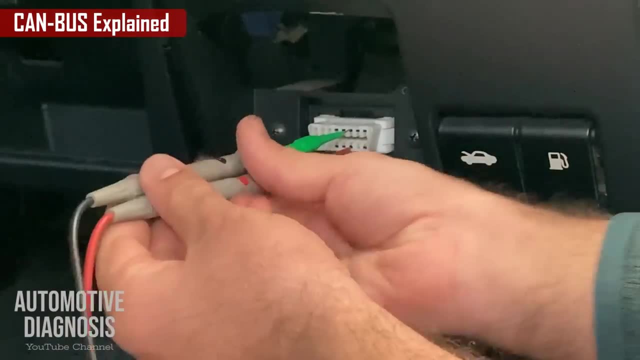 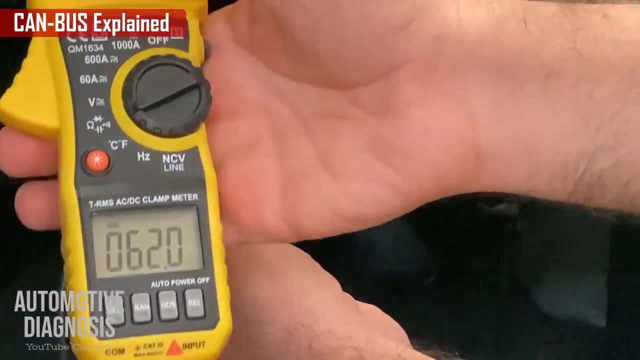 canvas from the obd2 connector, just as i did, uh, find pin number 6 and 14 and check the total resistance when ignition switch is off. so the total values should be something around 60 ohm. so already we have 62, which is acceptable, but you need to make sure ignition switch is. 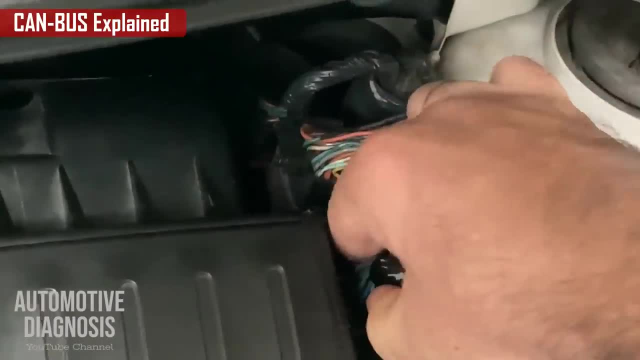 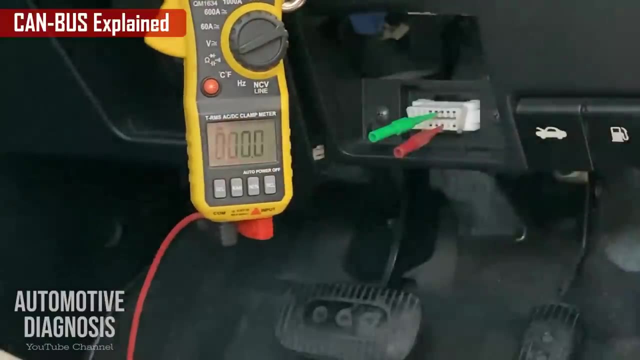 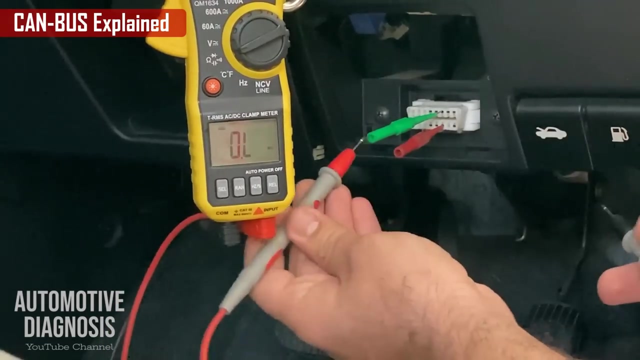 off. but what happens if one of the canvas uh resistance is? it's not working. so what i do? i remove the ecu engine ecm connector just to uh to disconnect the canvas resistance inside the ecm. and i'm going to check the resistance again and what i read here as a 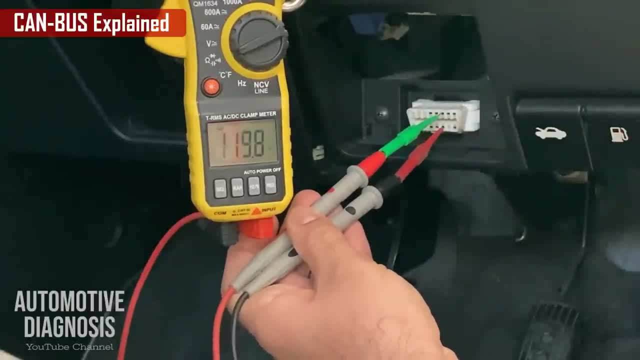 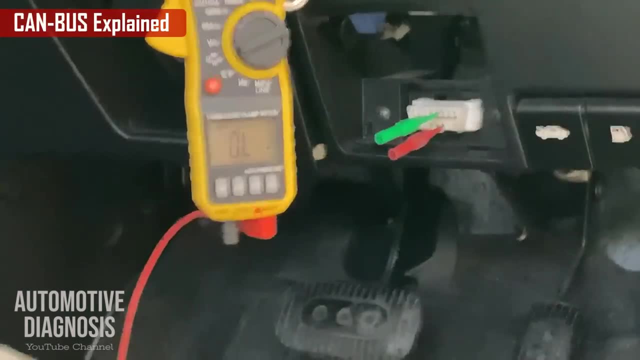 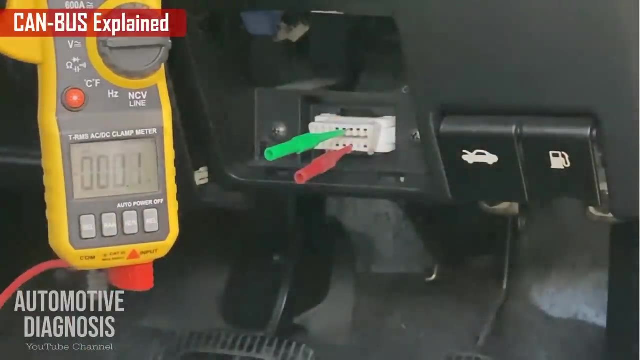 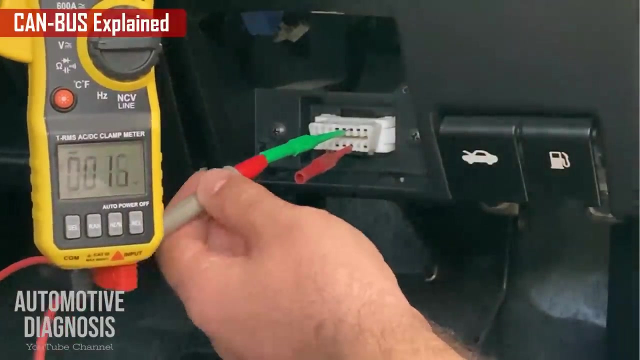 as you see, is going to be something around 120 ohms. so this value shows one of your canvas terminating resistor is not working. next step is going to be to check the voltage on the canvas. so what i do? i'm going to select the voltage on my multimeter and i go one by one. this time ignition switch must be on. i go one by one. i. 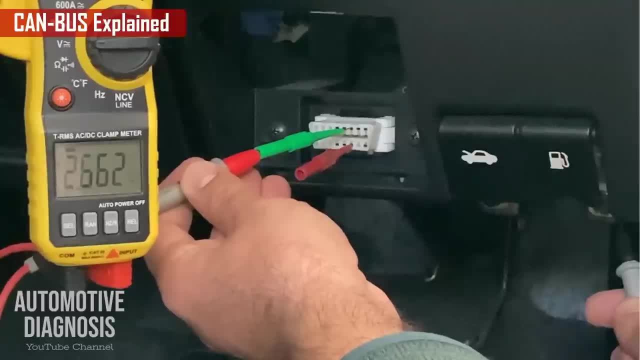 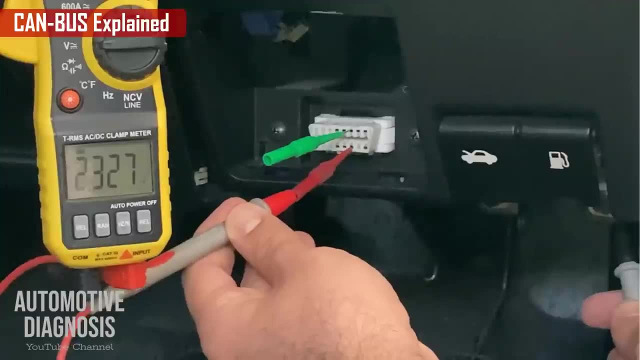 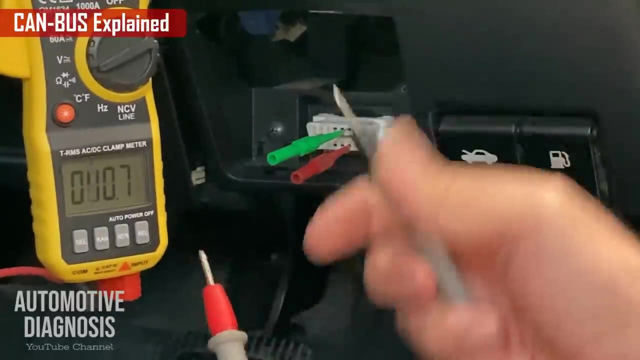 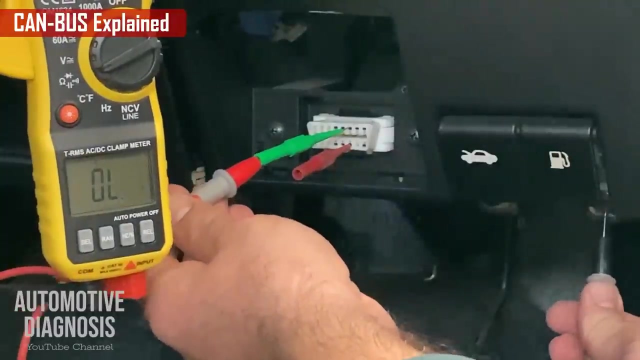 go two by one. and this is actually. if i click on it, it's lantern on the demand level, but that's National. and then i will now change my voltage level to hdw and wow, that is some amazing voltage. as you see, my jesteśmy on canvas hightle cable when i go down the node. that's playing a little. 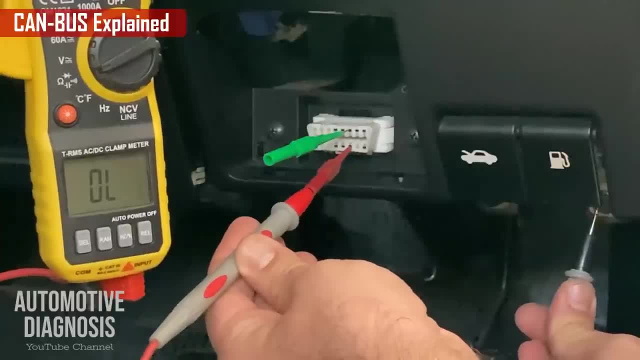 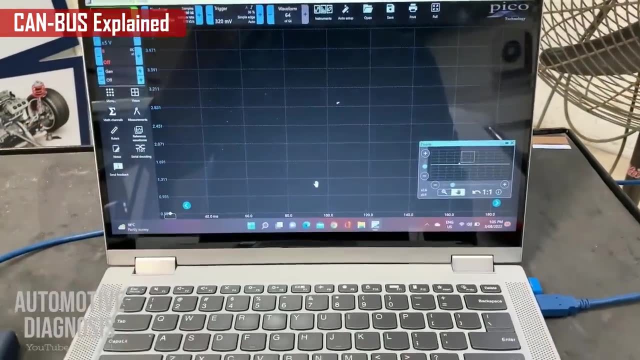 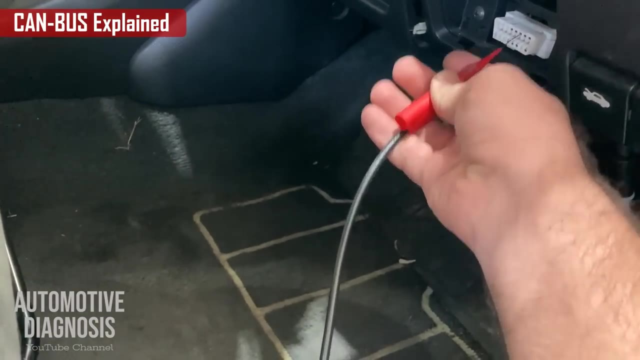 voltage back and forth in the data individually, one by one, and the other cable must be on ground. i shouldn't have any continuity during this test. next step is going to be reading the waveform using the pico scope. so what i'm going to do? i'm going to put the red prop on the canvas high and the black one should. 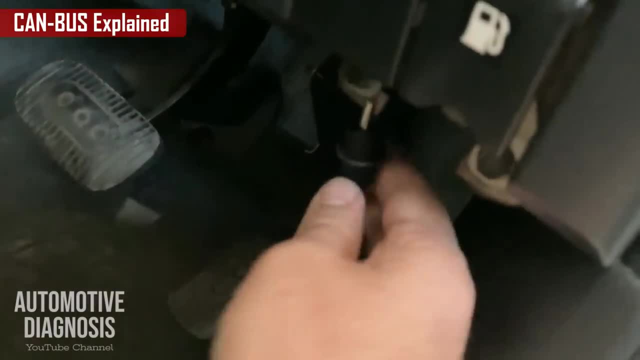 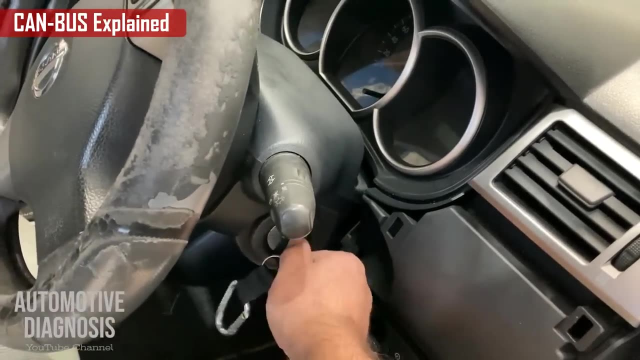 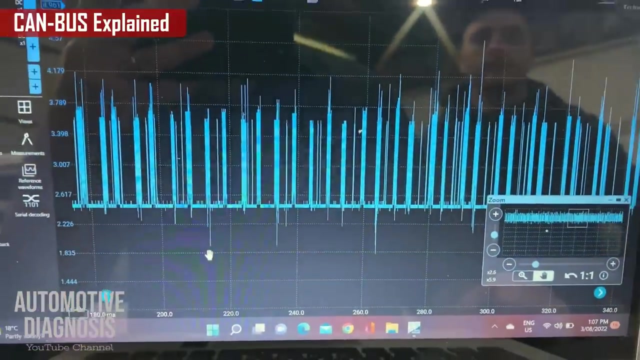 be connected to the ground and just to make sure that canvas is working, i'm gonna start the car to make sure all the units connected to the canvas are sending and receiving the information, so i'm gonna have a good waveform. so this is the waveform for the canvas: high. so, as you see, 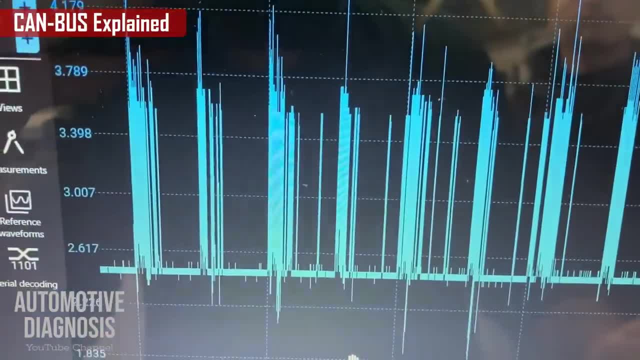 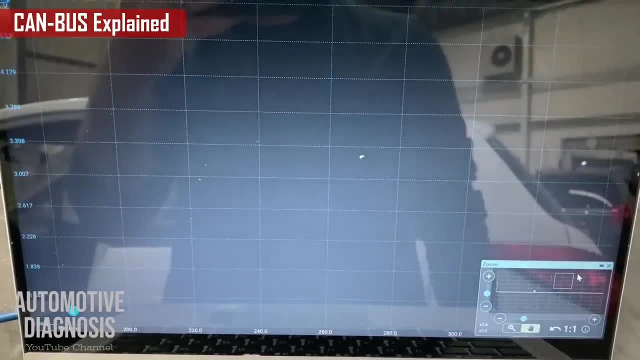 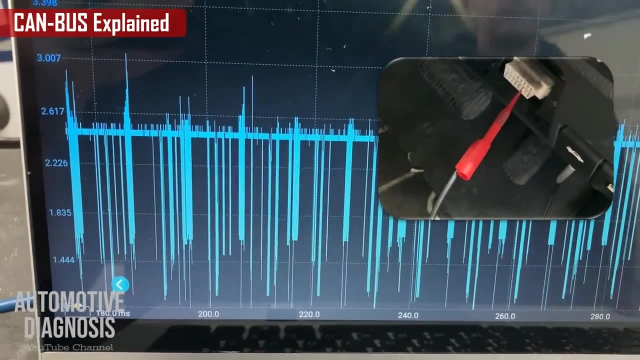 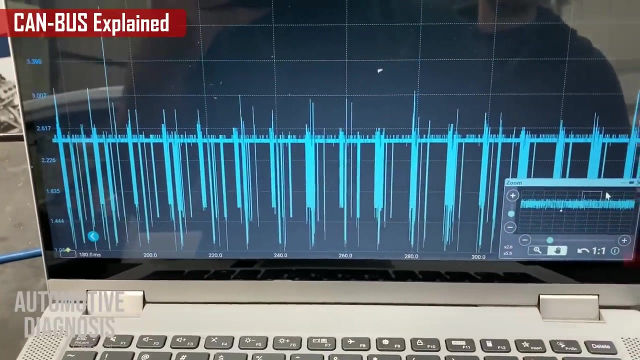 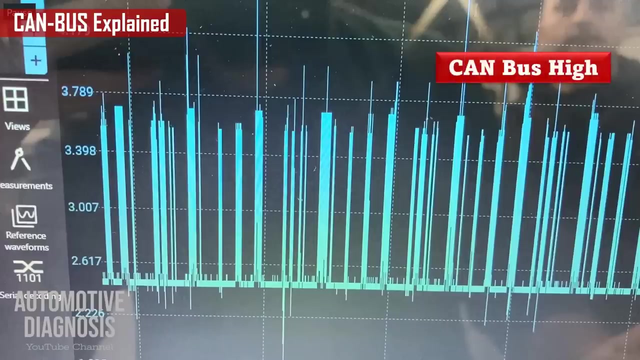 the waveform uh is changing from 2.5 to 3.5 volts and if i change uh- the red prop- to the canvas low, i'm gonna have the voltage dropping from 2.5 to 1.5 uh voltage. so here you see the value on the canvas high. i'm gonna have the voltage changing between 2.5. 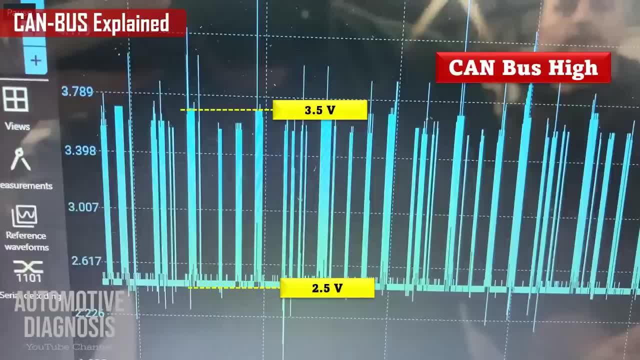 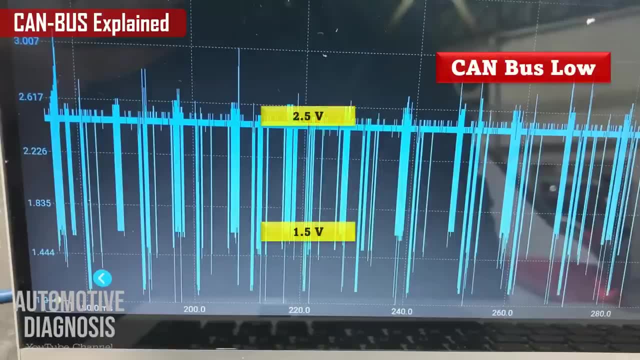 to 3.5 volt. this is what i get from the waveform on the canvas. low, my voltage is going to drop from 2.5 to 1.5. but what happens if i do have any short to ground on one of the canvases? i'm going to have the voltage drop from 2.5 to 1.5. 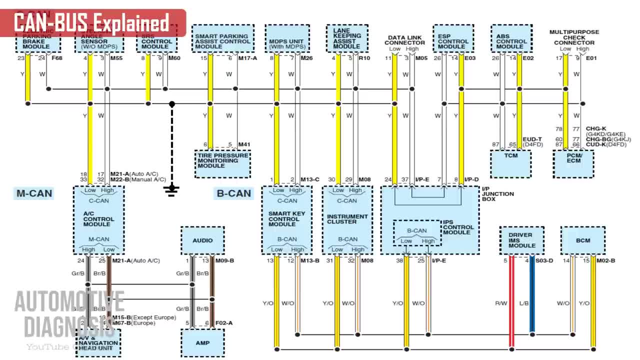 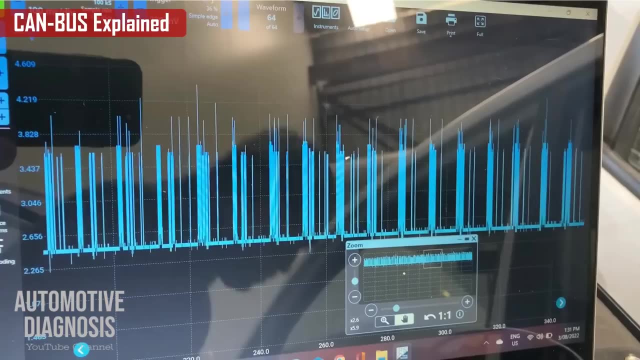 of those canvas wires, like the canvas high or canvas low. so of course i i won't have any communication. but what's going to happen to the waveform? so this is the canvas highway waveform when everything is normal. but as soon as i make the short to ground, you see the voltage is going.